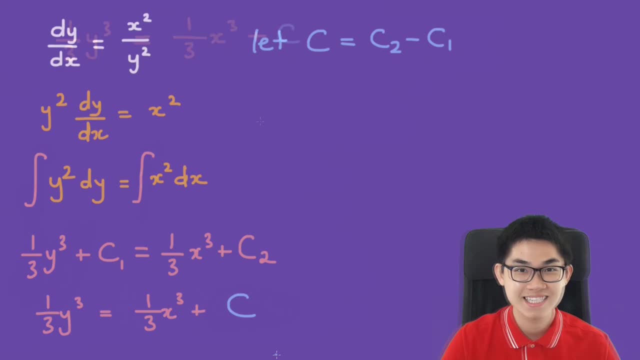 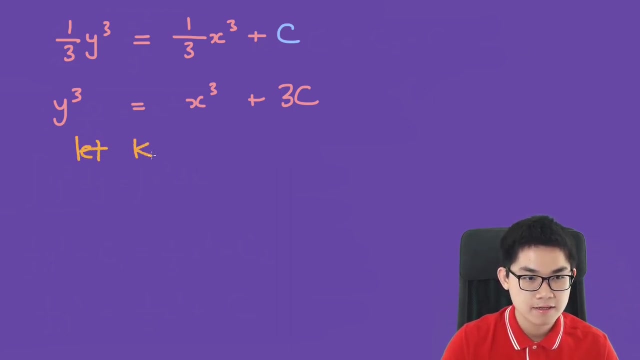 this whole expression and just simply write c. we will multiply both sides by 3 and we get y to the power of 3 is equal to x to the power of 3 plus 3c. and we'll also write let k equal to 3c, so we can replace this with a k. 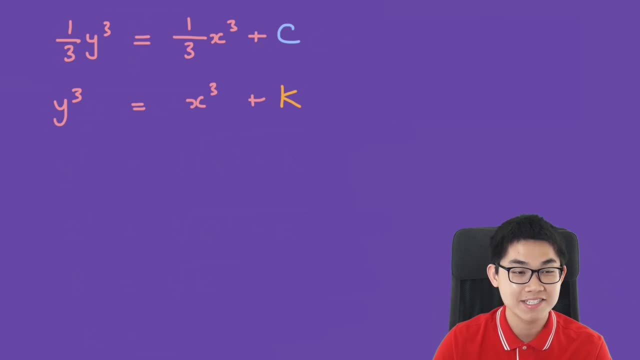 and finally we take the cube root of both sides, so we get: y is equal to the cube root of x, to the power of 3 plus k. so at this point, if you get this equation, then you're basically done. but let's say the problem also gives you an initial condition. then what do? 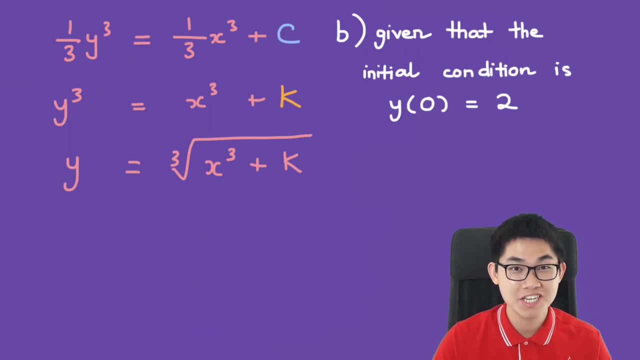 you do in that case, part b of the question asks you to fix the equation, given that the initial condition is: y at 0 is equal to 2, so what this means is: when x is equal to 0, y will be equal to 2, and let's just substitute this back into this equation, so we have: 2 is equal to the. 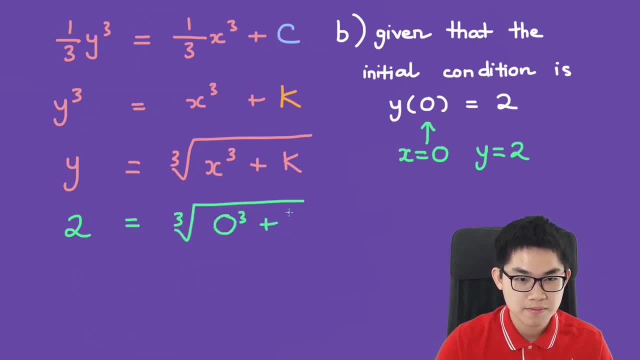 cubed root of 0 to the power of 3 plus k, so we have: 2 is equal to a to the power of 1 over 3, so k is equal to 8. we replace k with 8 and this is our final answer. 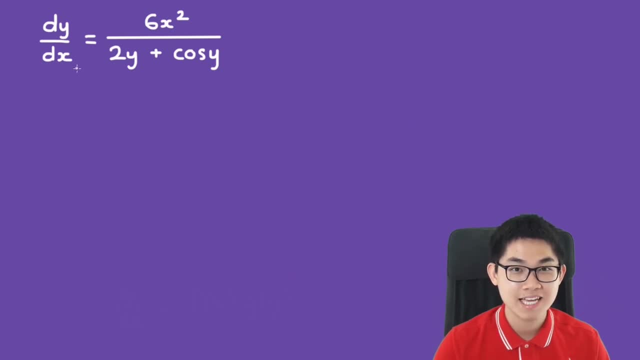 dy over dx is equal to 6x squared over 2y plus cosine of y. so again, let's bring all the y's to one side and the x's to the other side. we'll multiply both sides with dx, get dy is equal to 6x squared dx over 2y plus cosine of y. then we'll multiply both sides by 2y plus cosine of y. 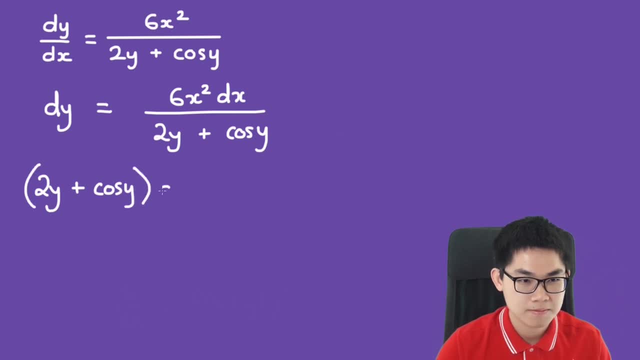 and this is equal to 6x squared dx. the next step is to integrate both sides. so we integrate both sides and here we have 2 times the integral of y dy plus the integral of cosine of y dy, and that's equal to 6 times the integral of x squared dx. so notice, we can bring the. 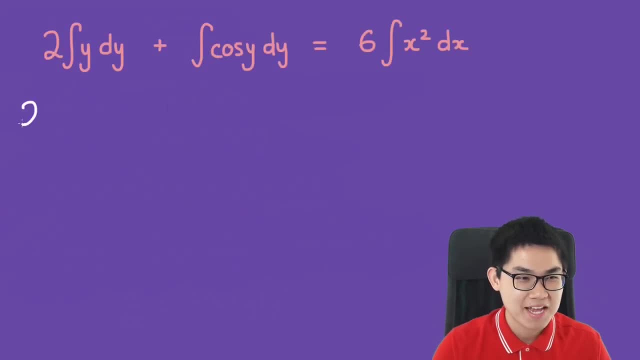 conon to the right and the conon to the left, so we can bring the conon to the left and we get the entire constant outside of the integral. we get 2 times 1 over 2 times y to the power of 2 plus c, but let's write that later. then, plus what is the integral of cosine of y? 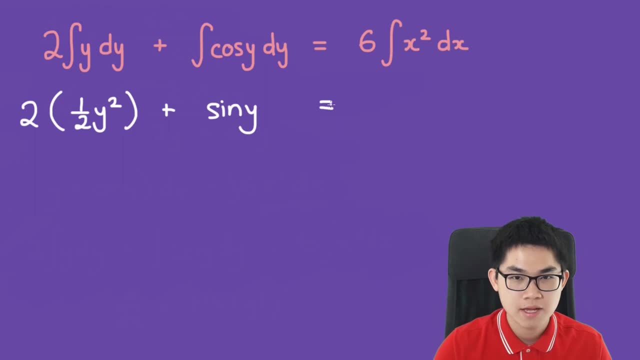 well, it's going to be sine y, and here we have 6 times 1 over 3, x to the power 3. so i know, over here we have plus c2, over here we have plus c1, and then we bring all of them to one side, and so 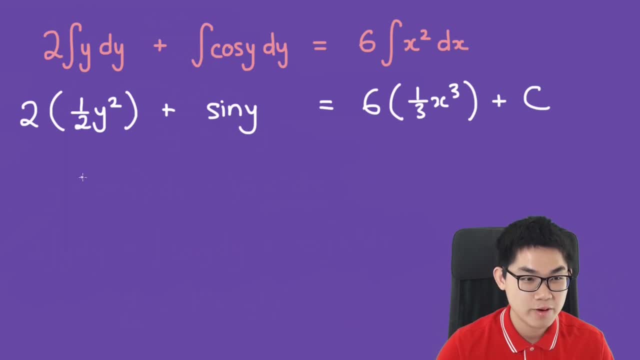 we'll have 2 times 1 over 2 times x to the power 3. so i know, over here we have plus c2, over here we have have c, like this, and finally we will have y squared plus sine y and that is equal to. 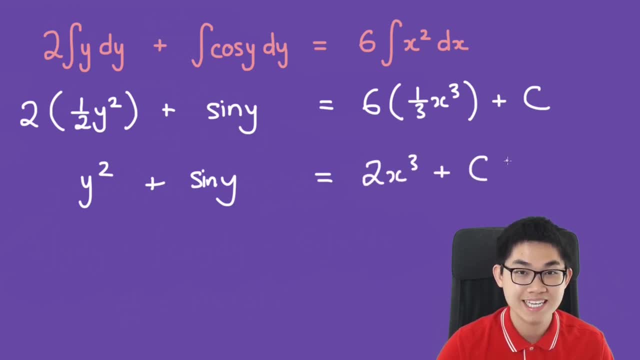 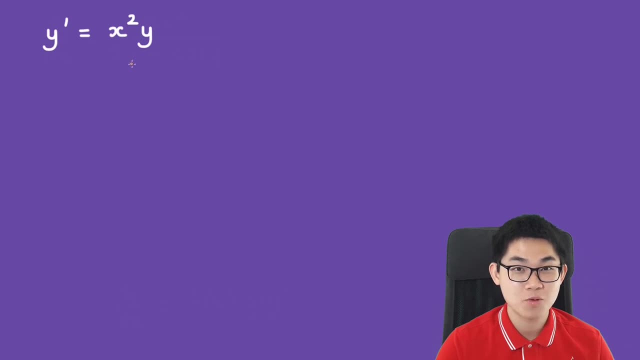 2 times x to the power of 3 plus c. and this is our equation: y prime is equal to x squared times y. so whenever you see a y prime, just turn it into dy over dx. so we have dy over dx is equal to x squared times y. and then we divide both sides by y. we get 1 over y, dy over dx. 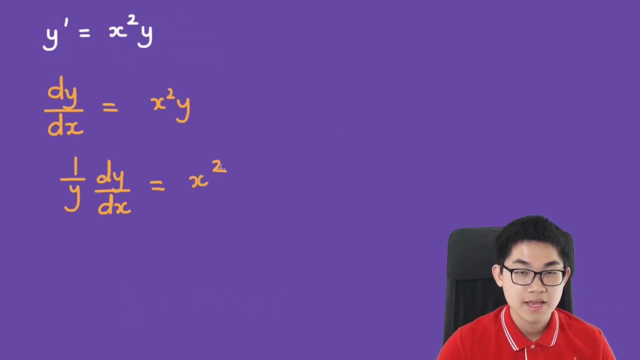 is equal to x squared, and then multiply both sides with dx, you get 1 over y. dy is equal to x squared dx. now one mistake that a lot of students might make is that when they divide both sides by y, they will just say y is not equal to zero. but that might not be true. 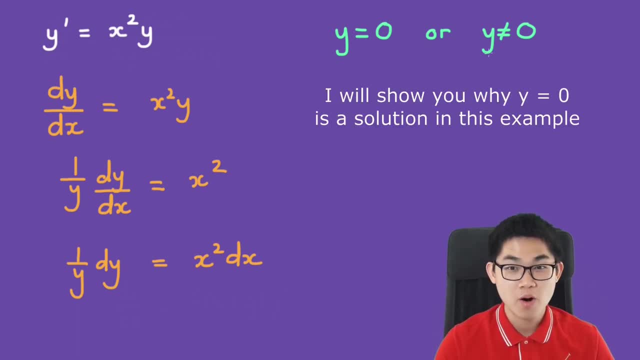 you have to check: can y be equal to zero or y is not equal to zero? now let's try. let's try: y is equal to zero. so if y is equal to zero, then y prime, or the derivative of y, is equal to zero, is also zero. and then we substitute this back into this equation. so y prime is zero. we have 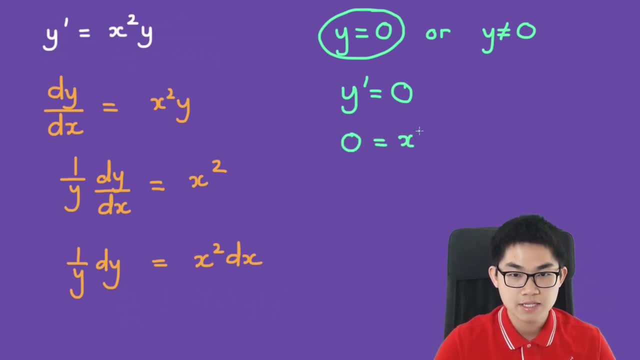 zero on the left side and that's equal to x squared times. y and y is also zero. so we get: zero is equal to zero and since this equation is true, y can be equal to zero, and it is a solution- we're going to integrate both sides. so what is the integral of 1 over y? dy well, 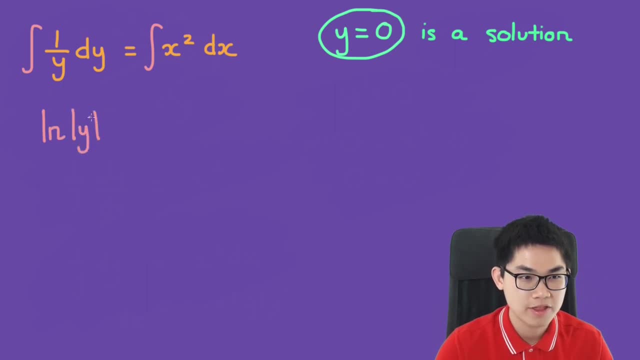 it is going to be the ln of y with the absolute value, and that's equal to 1 over 3, x to the power of 3 plus c. so at this point i'll show you a trick to solve this equation: you just take e to the. 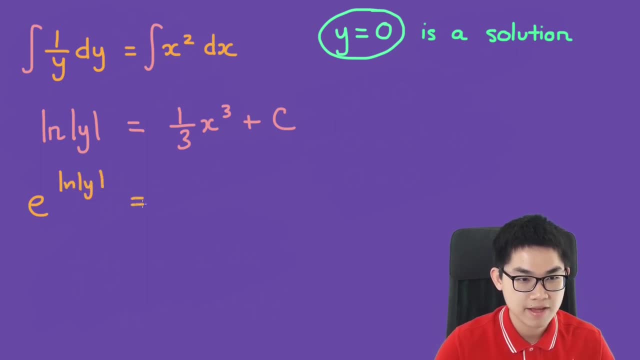 power of ln, y and the same thing on the right side: e to the power of 1 over 3, x to the power of 3, plus c, e to the power of ln. absolute value of y. it's just the absolute value of y. and on the right hand side, we have e to the power of 1 over 3, x to the power of 3. 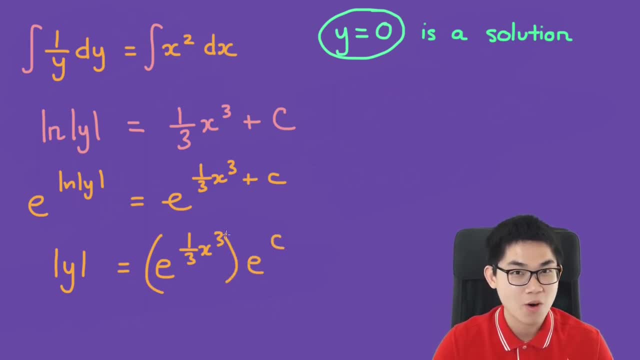 and this whole thing times e to the power of c. and why is that the case? well, if you remember from high school, there is a formula. but when you have, let's say, a to the power of b plus c, then this is equal to a to the. 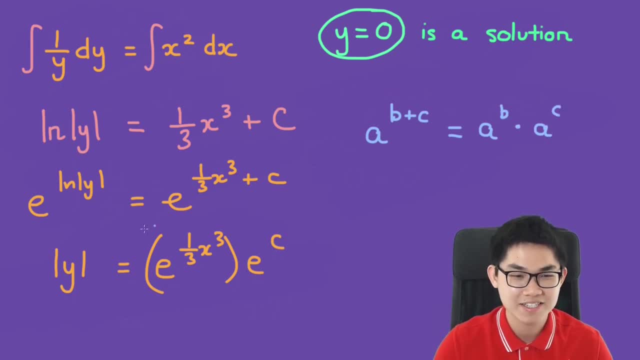 power of b times a to the power of c, and hence that's why we're writing it like that and we're almost done. so what we want to do here is get rid of the absolute value, and if you remember, let's say we have the absolute value of x is equal to 2, that x will be equal to. 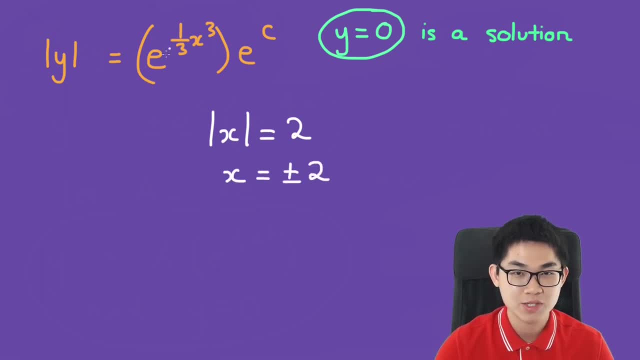 plus and minus 2, and that's what we're going to do here as well. y is equal to plus and minus to the power of c times e to the power of 1 over 3, x to the power of 3, so you can leave it like: 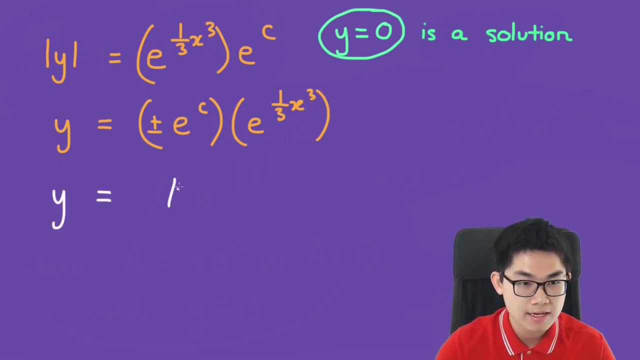 this: or you can also say y is equal to a. I'm just going to pick a letter: a times e to the power of 1 over 3, x to the power of 3 where a is equal to 0, because again, y can be equal to 0 or a can be. 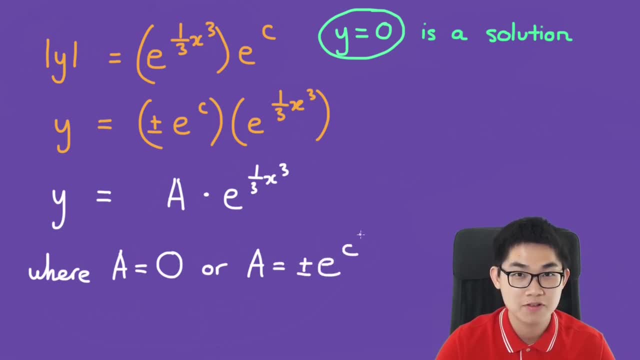 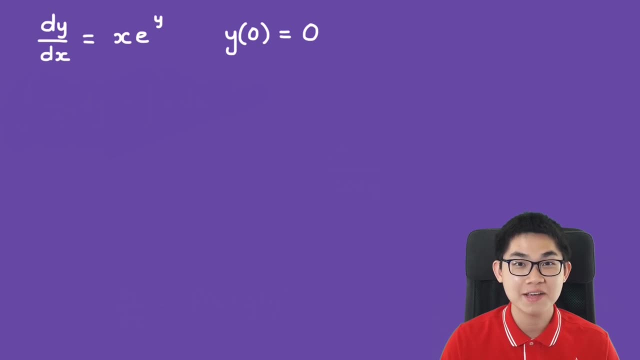 equal to plus and minus e to the power of c. so this whole thing right here is your solution. one last problem for today: we have dy over dx is equal to x times e to the power of y, and we're also given the initial value: y at 0 is equal to 0, so go ahead and pause this video. 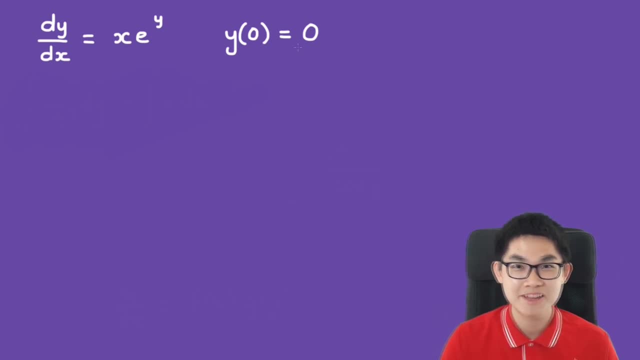 and give it a try, and then we'll go through this together. are you ready? okay, now let's move all the y's to the power of c and we're also given the initial value. y at 0 is equal to 0, so go ahead. one side and the x to the other side. we will start with multiplying both sides by dx. we get dy is. 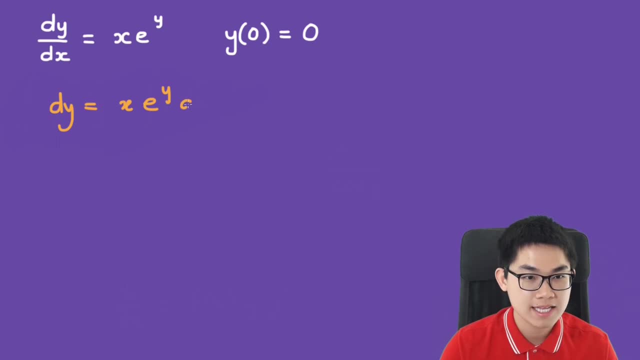 equal to x times e to the power of y times dx. and then we divide both sides by e to the power of y, so we have 1 over e to the power of y. dy is equal to x times dx. now, instead of writing 1 over e to, 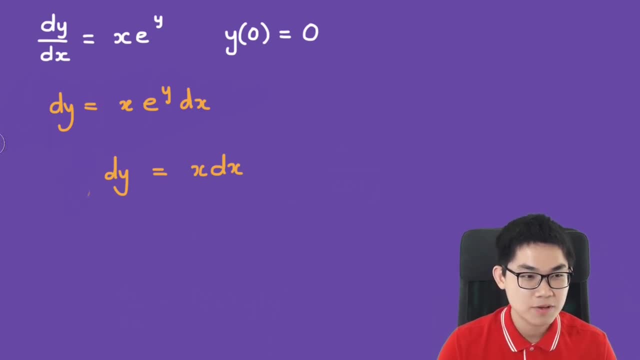 the power of y. i'm just going to write e to the power of negative y. it means the same thing. we're going to integrate both sides. let's solve this one first. so which method should we use for this one? well, it has to be the u substitution, right. we have let u be equal to negative y. we take the. 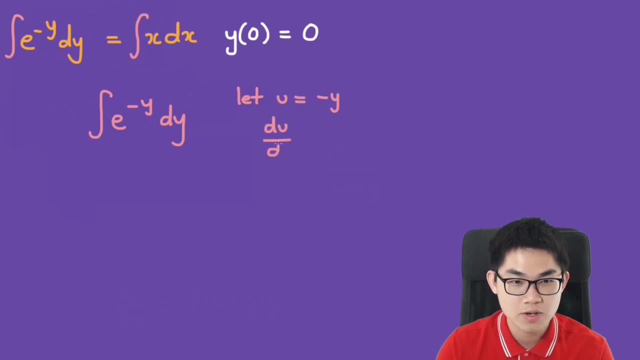 derivative of both sides. so du over dy and that's going to be equal to negative 1. so du is equal to negative dy and dy is equal to negative du. now let's fix this one. so we have the integral of e to the power of u and dy is equal to negative du. we have negative the. 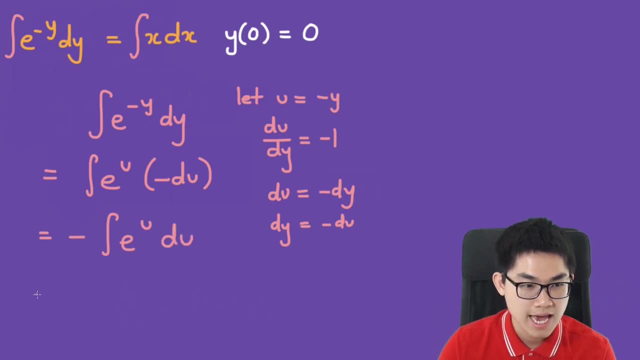 integral of e to the power of u du, and this is equal to negative e to the power of u plus c, and we need to replace u with negative y. How about the right-hand side? What is the integral of x- dx? Well, that's going. 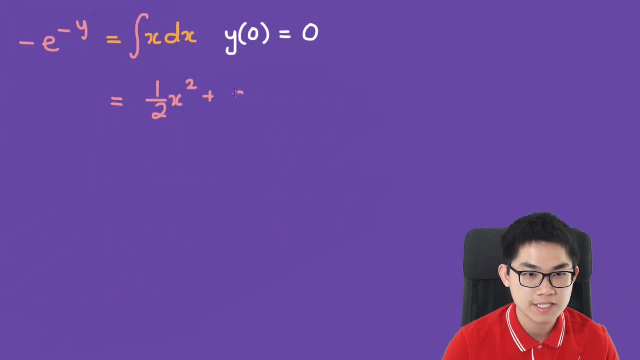 to be 1 over 2, x to the power of 2 plus c. At this point we can substitute the initial value into the equation to find c. So this here means, when x is equal to 0, y is equal to 0. And let's go ahead.